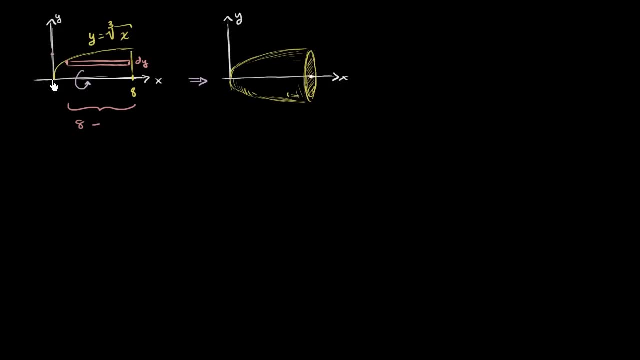 We're going to be integrating with respect to y over an interval in y. And so we really want to have everything in terms of y. So this x-value, whatever it is, as a function of y. So if y is equal to the cube root of x, we can cube both sides. And we could get x is equal to y to the third power. These are equivalent statements right over here. And so this distance right over here is going to be 8 minus y to the third, if we were to express it in terms of y. 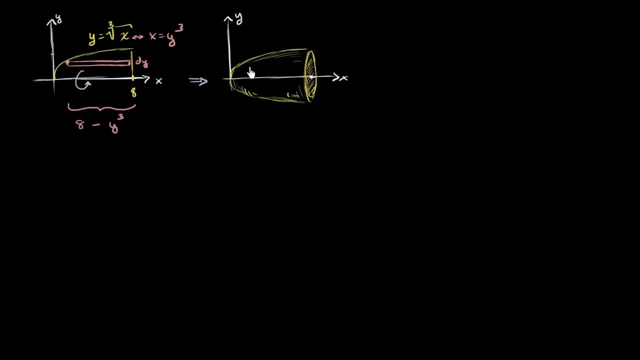 And then when you rotate that thing around the x-axis, it's going to construct the outside of a cylinder, or a shell, as we like to call it. And I'll try my best to draw that shell. So it will look something like this. 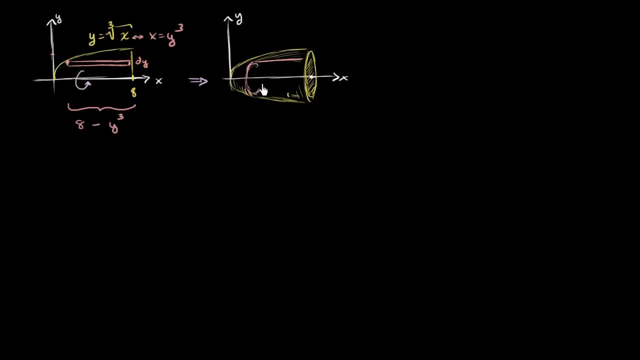 So you're going to have a shell that looks like this. And there you go. And then actually, this shares a common boundary right over here. So you're going to have a shell that looks something like that. 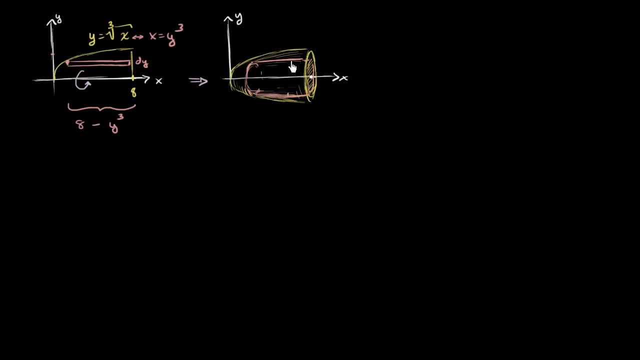 So that hopefully helps a little bit. Let me give it some depth. 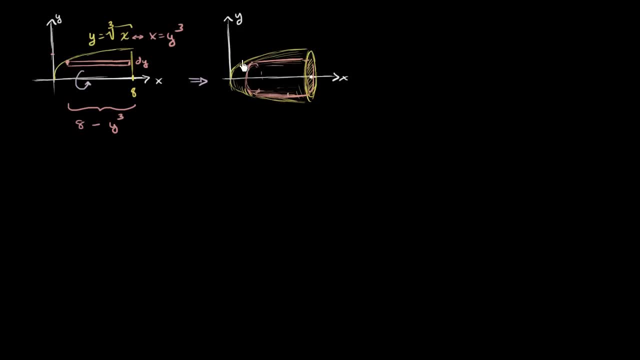 So you'll have a shell that looks something like that. And if we could figure out the volume, the volume of that shell, which is really going to be the volume of the outer surface area times, or the area of the outer surface area times the depth. And then if we were to sum up all of those shells, this shell is for a particular y in our interval. 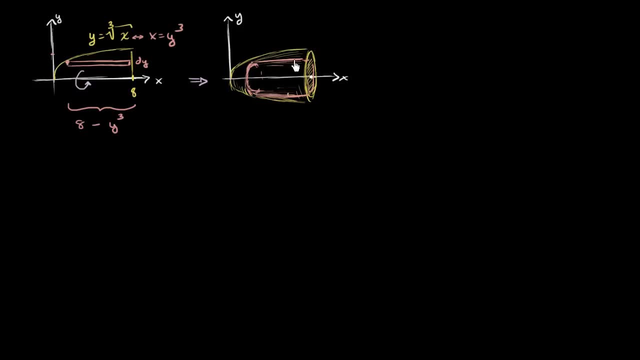 If we were to sum up over all of the y's in our interval, all of the shells, all the volumes of the shells, then we have the volume of this figure. 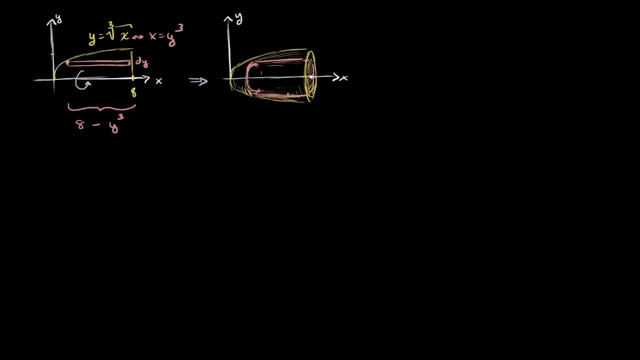 So once again, how do we figure out the volume of a shell? Well, we can figure out the circumference of kind of the top, or I should say, the volume of the shell. I guess the left or the right, in this case. The left or the right of our cylinder. If we can figure out that circumference, circumference is equal to 2 pi times the radius. And what is the radius? 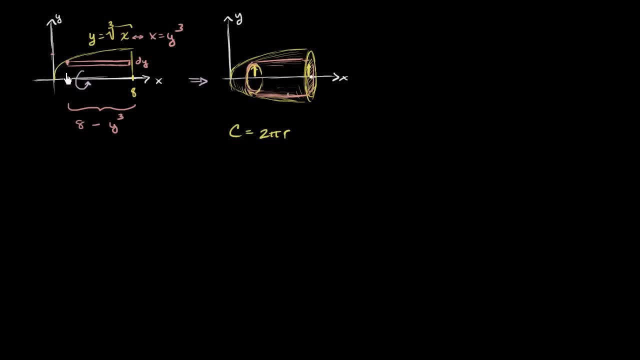 The radius of these things are just going to be your y value. That's this distance right over here. That's just going to be the y value. 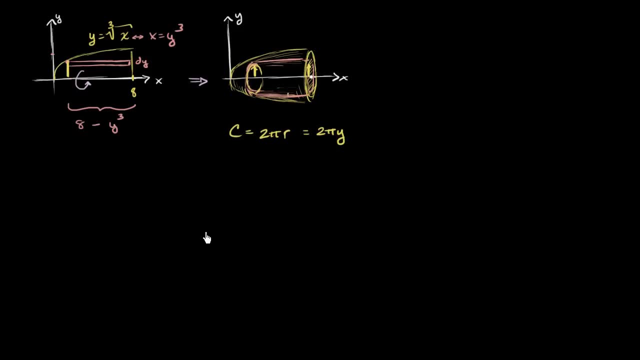 So it's going to be equal to 2 pi times y. And then if we want the area of the outer surface, we just multiply that, the circumference, times the width of our cylinder. So let me write it over here. 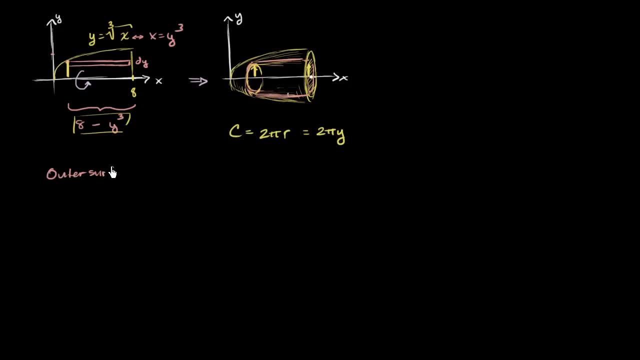 So outer surface area is going to be equal to our 2 pi y times our 8 minus y to the third. 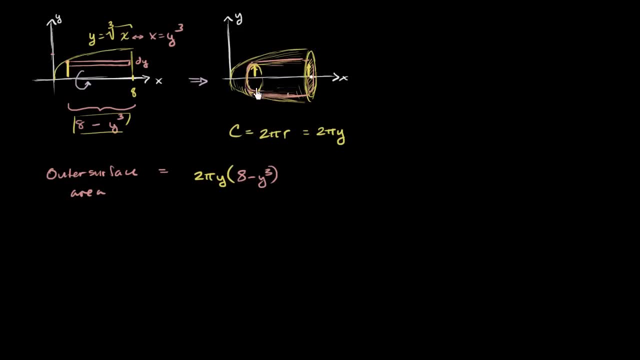 8 minus y to the third is just this length. You multiply that times circumference, you get the outer surface area. 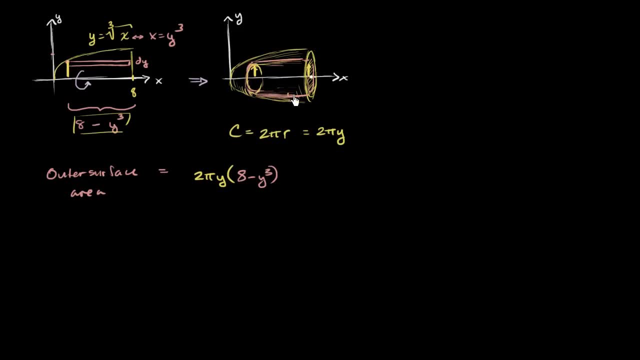 Now, if you want to find the volume of this one shell, it's going to be the outer surface area, 2 pi y times 8 minus y to the third, times the depth. Times this dy right over here. Times the dy. I'll do the dy in purple. 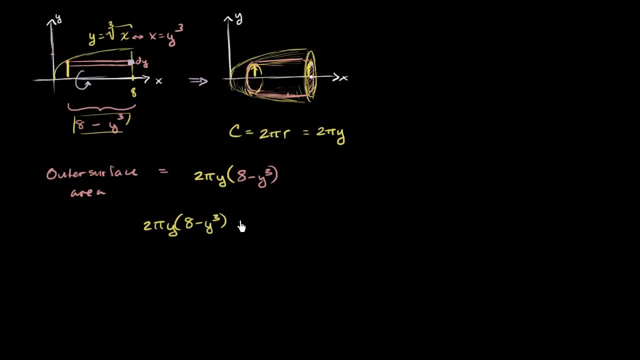 Times the dy. Times the dy. So that's the volume of one shell. 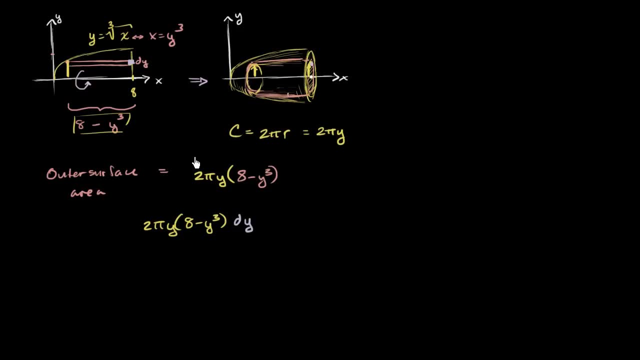 If we want to find the volume of the entire, solid of a revolution, we have to sum all of these up. And then take the limit as they become infinitely thin, and we have an infinite number of these shells. 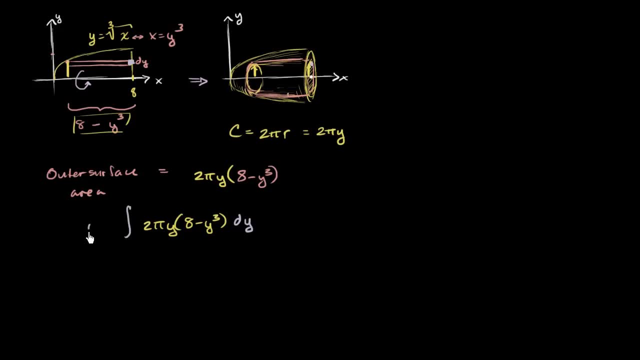 So we're going to take the sum from, and remember, we're dealing in y. So the volume is going to be equal to. So what's our interval in terms of y? So y definitely starts off at 0. And when x is equal to 8, what is y? Well, x to the 1 third power is just 2. So y is 2. This value right over here. Let me make it a little bit clearer. This value right over here. This value right over here is 2. So y goes from 0 to 2. 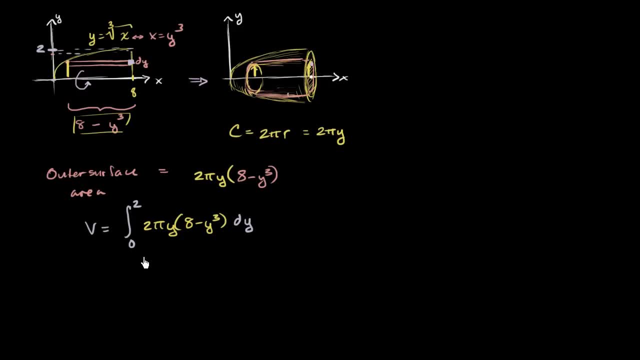 And we've set up our integral. And this one looks pretty straightforward. So I think we can crank through it in this video. So this is going to be equal to. We can take out the 2 pi. 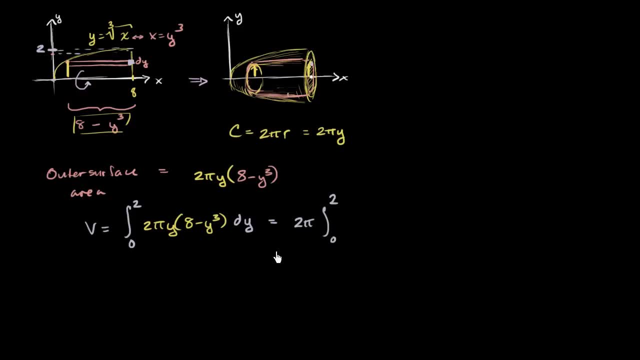 2 pi times the definite integral from 0 to 2 of, let's multiply the y, of 8y minus y to the fourth. All of that dy.